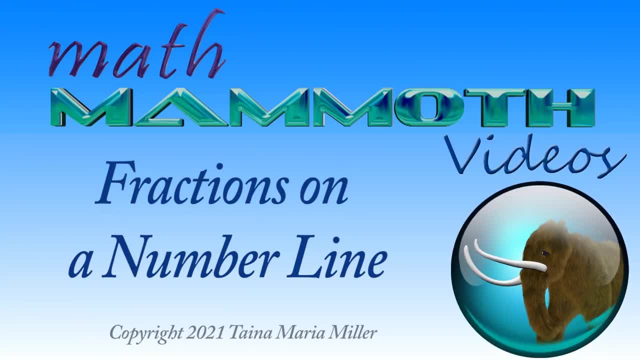 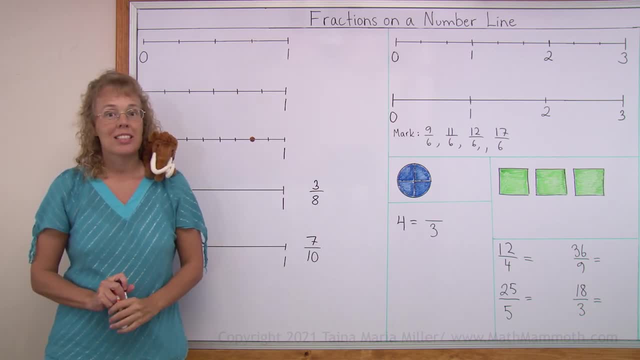 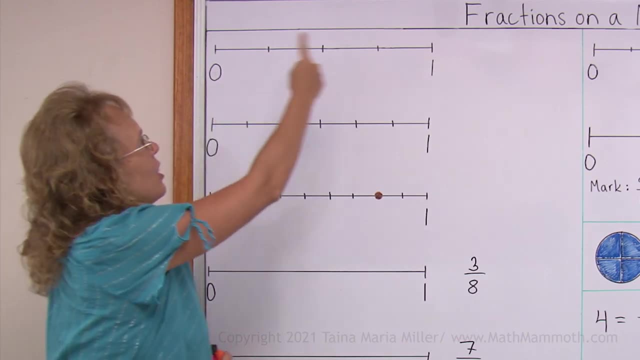 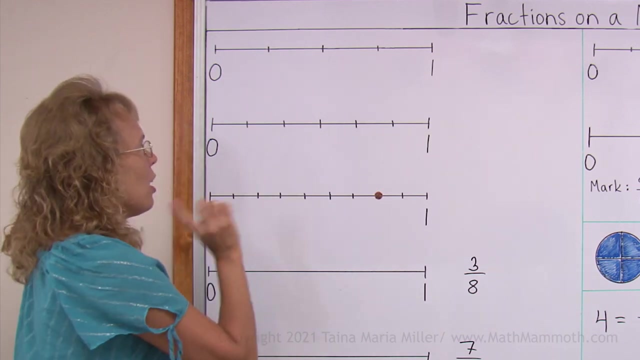 Hello, my name is Maria and this is Matthew, my mascot. In this lesson we're gonna study fractions on a number line. First of all, I have a number line from 0 to 1, and how many parts is it divided into? Now do not count 3 tick marks and say 3, because it is not divided. 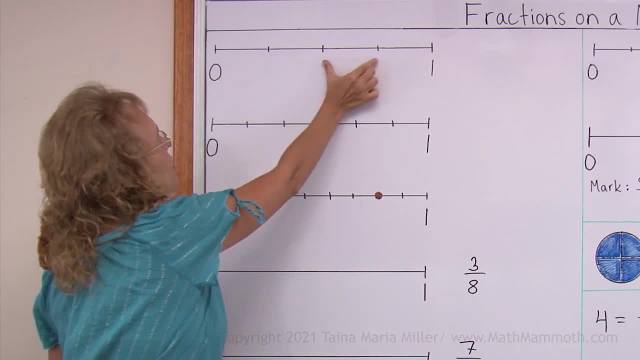 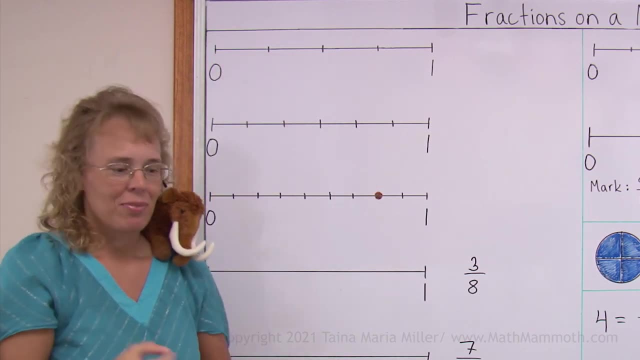 into 3 parts. It is divided into 1,, 2,, 3 and 4 parts. That's how you need to count the parts. okay, Like units here. So 4 parts And therefore we can mark the fractions 1. 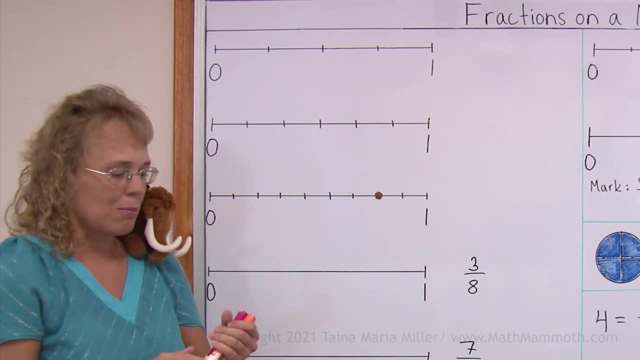 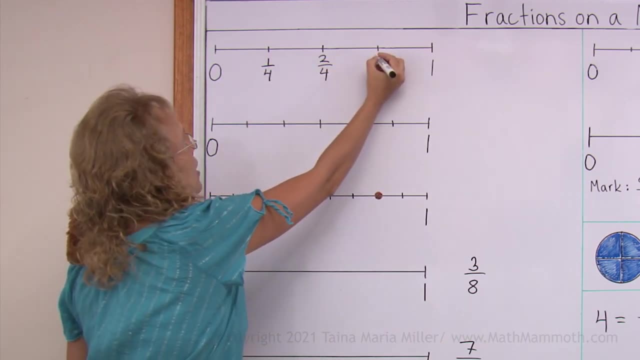 fourth, 2 fourths and 3 fourths on that number line. This tick mark is for 1 fourth, The next one 2 fourths and this one is 3 fourths. This one is the same as 4 fourths. 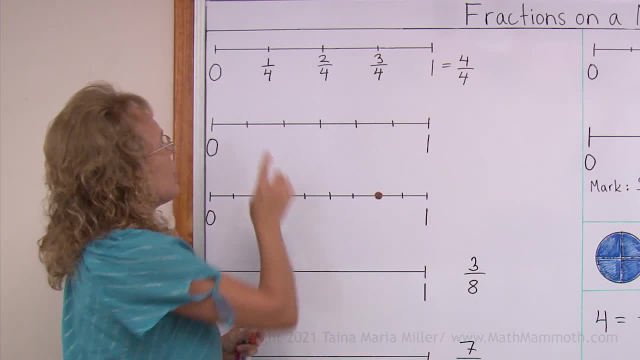 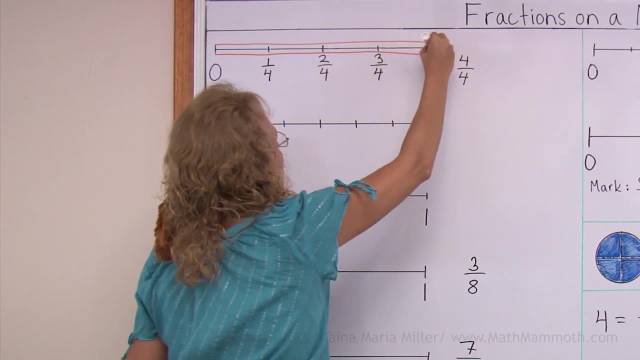 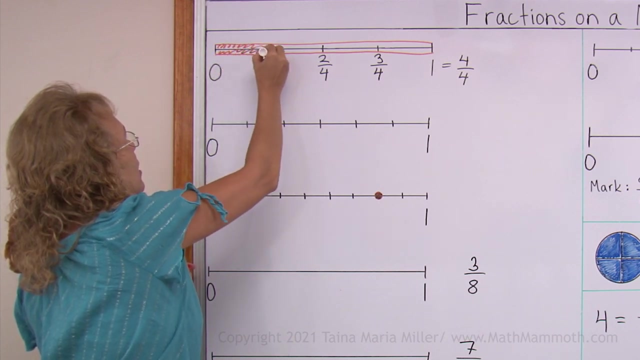 Or 1 whole. okay, If you don't see it, think of it as a rectangle like this: If this was a long, skinny rectangle and then you would divide it into 4 parts and then you would color, say, 1 part. If you color 1 part, you reach up to 1. fourth, the tick mark for 1. 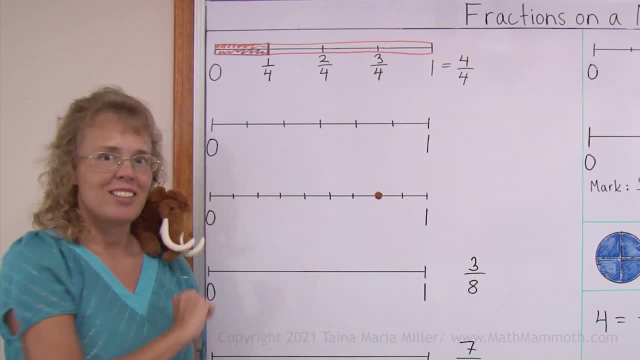 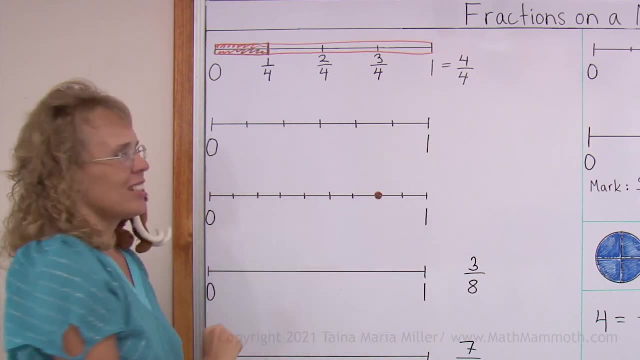 fourth: okay, Now this number line. how many parts is it divided into? Okay, we're gonna count. Well, I can't count the tick marks 1,, 2,, 3,, 4, 5 and say I cannot say 5.. I can. 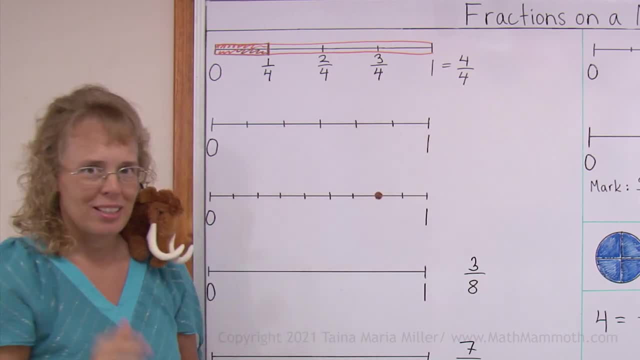 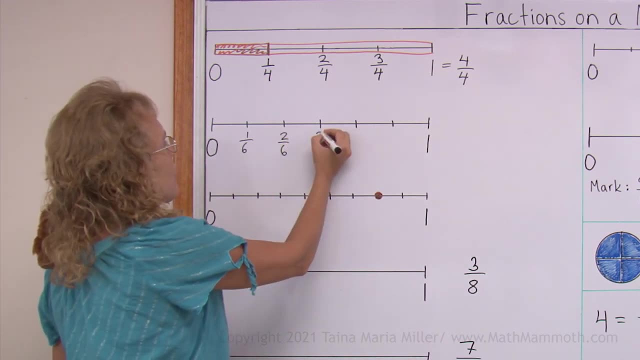 count this way: 1,, 2,, 3,, 4,, 5,, 6.. 6 parts. So when we come to this tick mark, it is 1- sixth, And then 2 sixths, 3 sixths, 4 sixths, 5 sixths, And then this tick mark is the same. 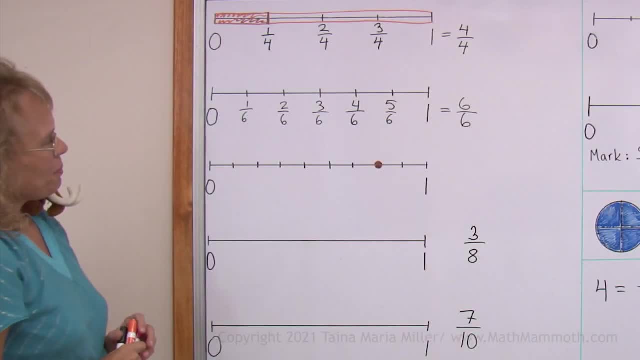 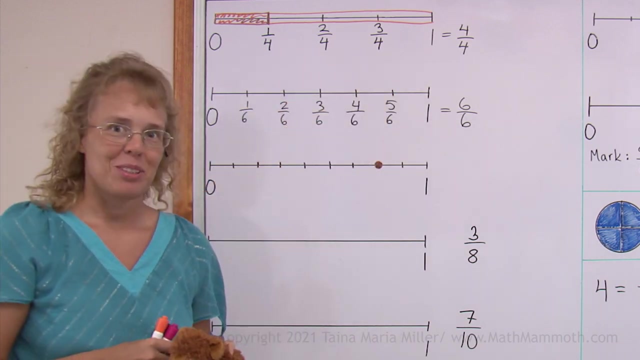 as 6 sixths. Now can you tell me what fraction does this dot mark? Oh, Matthew's saying No. he's not saying the answer. He says he wants to jump on the number line. You know Matthew likes jumping on number lines. He took 7 jumps and then.